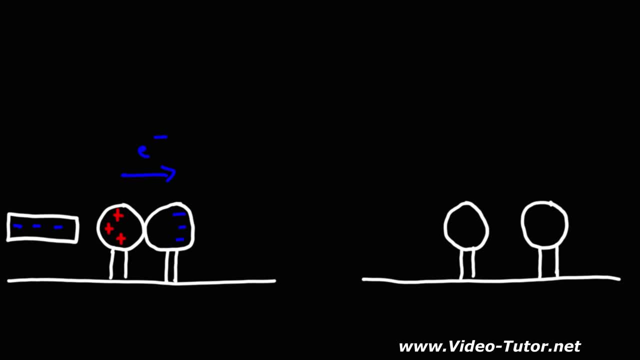 it's going to develop a net positive charge. Now let's say we take this sphere and move it to the right, So we disconnect these two metal spheres, and then afterward, once we disconnect them, let's remove the negatively charged metal rod. 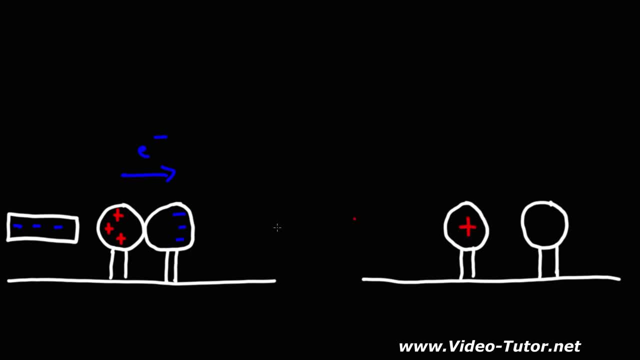 Once we do that, the sphere on the left is going to have a net positive charge, The sphere on the right, it's going to have a net negative charge, And so that is charging by induction. We were able to charge these two metal spheres using another charge object. 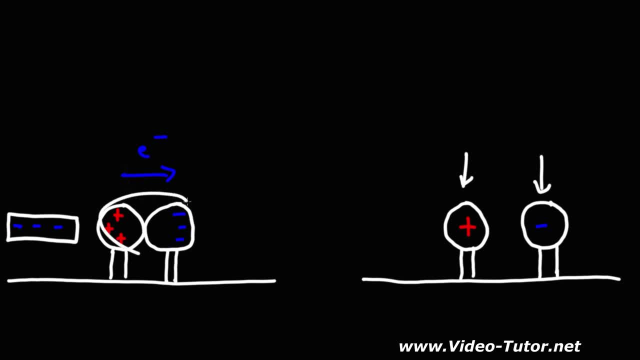 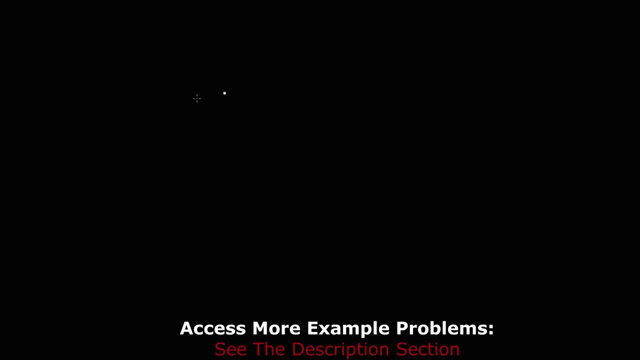 but there was no contact involved between these two metal spheres, the negatively charged metal rod. So that's charging by induction. It's when you have a charged object and you use it to induce a charge in another object without the charged object touching the neutral object. Now let's consider: 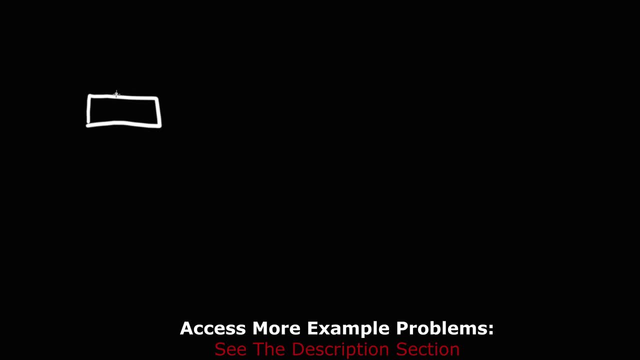 another example. So let's say we have a neutral metal sphere, just like before, but this time we only have one metal sphere, not two, and we're going to have a negatively charged metal rod. Now, as we bring this negatively charged metal rod closer to the metal sphere- the electrons in the metal sphere they're going to be. 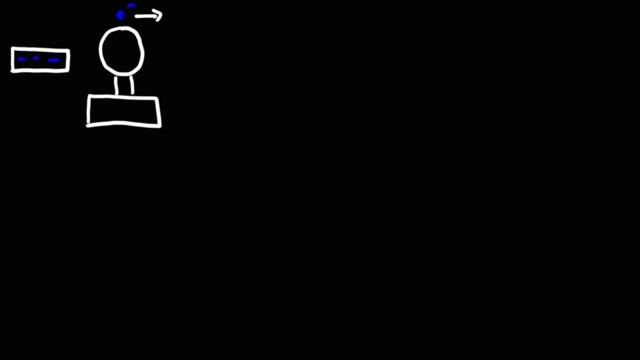 repelled and so they're going to move to the right. So on the right side we're going to have a buildup of negative charge. on the left side It's going to be electron-deficient, so the left side is going to have positive charge Overall the metal sphere. 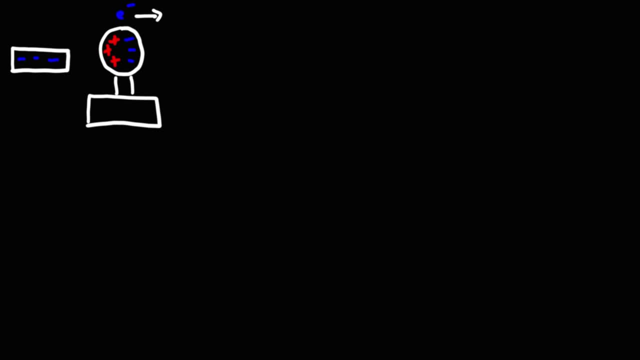 is still neutral. but notice that we have separation of charge. One side is positive, the other side is negatively charged. So at this point it's said that it can be said that the metal sphere is polarized due to that separation of charge. Now, what we're going to do at this point is we're going to take a metal wire.